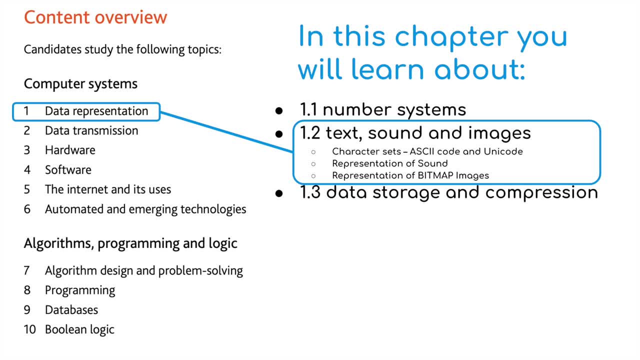 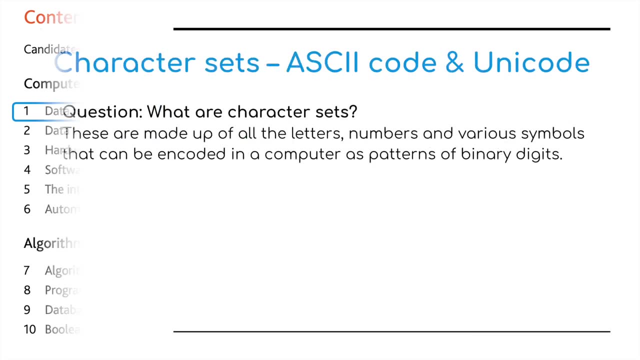 All these different file formats- text, sound and images- need to be converted into a binary format in order for a computer to understand and be able to work with it, and this video, hopefully, will explain all of that to you. So we start off with character sets, ASCII code and Unicode. but the question is: what are character sets? 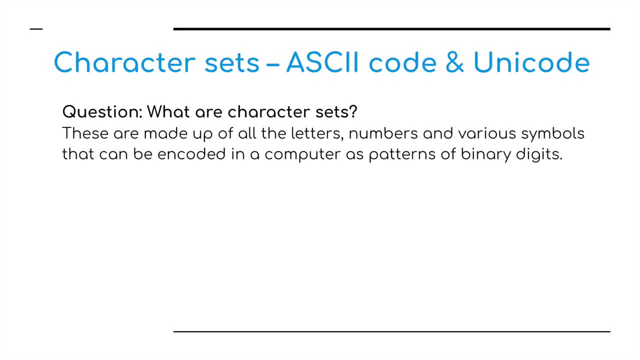 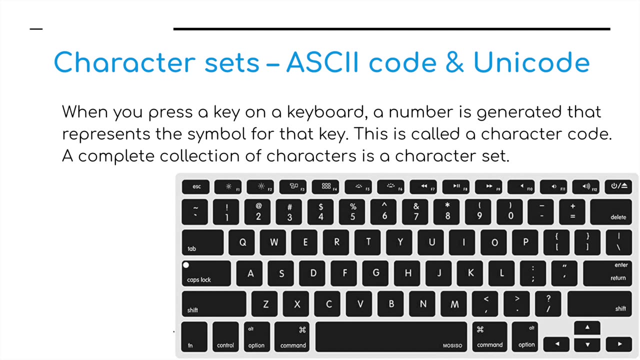 Well, these are made up of all the letters, the numbers and various symbols. They can be encoded inside a computer as patterns of binary digits. But what does that mean? Well, when you press a key on your keyboard, a number is generated that represents a symbol for that particular key. 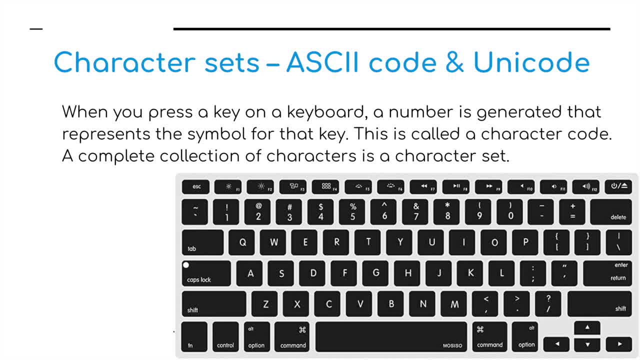 This is called a character code. A complete collection of characters is what's known as a character set. Now, what do I mean by that? For example, if we press the A- the capital A- on on your keyboard and the number 65 is generated, 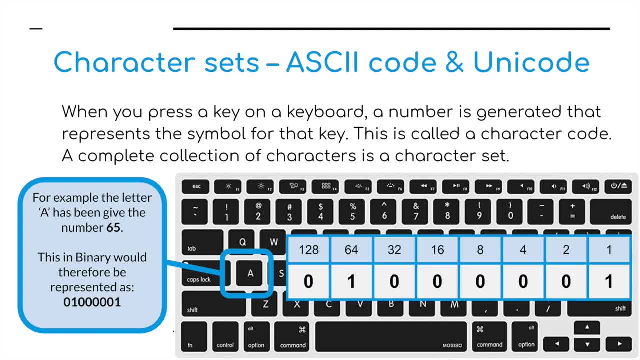 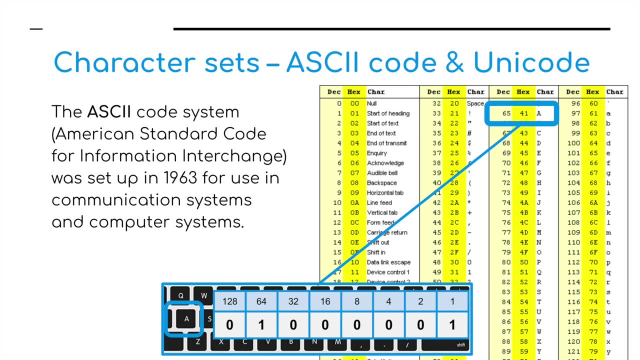 Now this, of course, is the denary number and that is converted into binary, which would be 01, one lot of 64, 00, 000, and then 1 being the 1, so 65.. The ASCII code system, the American Standard Code for Information Interchange, was set up a long time ago, back in 1963. 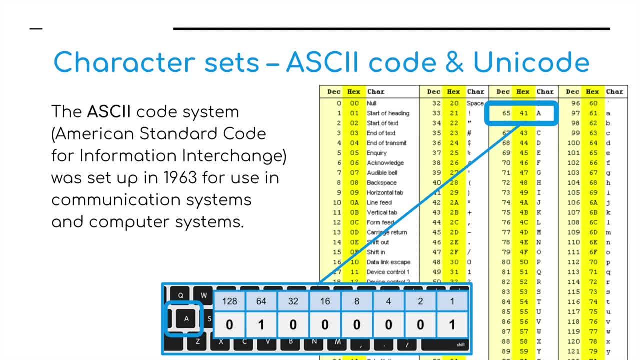 It was used for the use in the communication systems and the computer system. As you can see here, I've highlighted the character capital A on the keyboard, which has a decimal value of 65 and an hexadecimal value of 41, and of course that's been converted into binary, as you can see there. 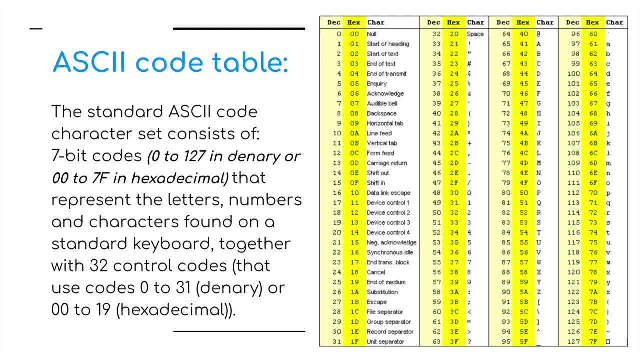 The standard ASCII code character set consists of seven bits, seven bit codes. So any number from 0 to 1 is set to 0. So any number from 0 to 1 is set to 0. So any number from 0 to 1 is set to 0. 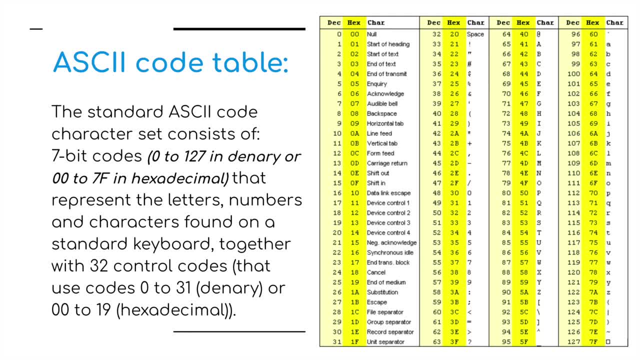 0 to 1 is set to 127 in denary, or 00 to 7F in hexadecimal. So basically, it allows for 128 different characters to be represented, characters that you can find on your standard keyboard. Also, together with that, 32 control codes moving from 0 to 31.. 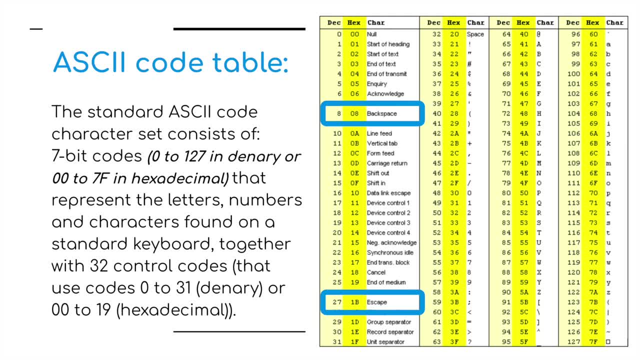 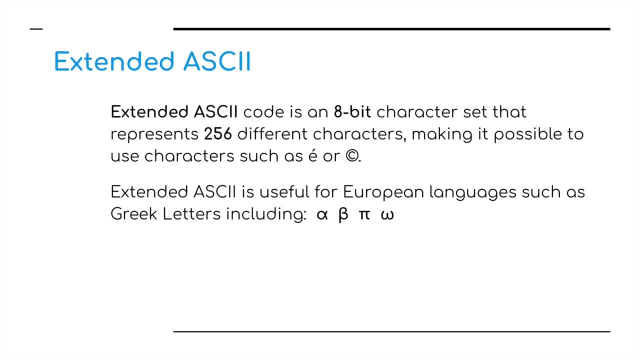 And, as you can see there, the backspace is represented by the number 8. and the escape key on the keyboard is represented by the number 27, or an x-decimal 1B. Now, obviously, 128 characters doesn't give us a lot of. 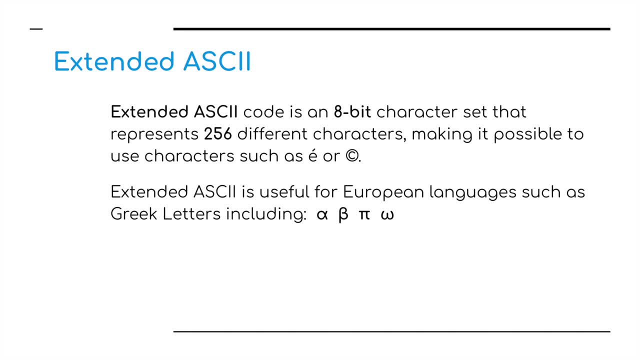 scope for storing numbers, symbols, letters, etc. so in the 1980s a version of ASCII came out, called Extended ASCII, which allowed for not 7 bits but now 8 bit character sets and doubling the number from 128 to 256 different characters. This enabled the storage of such characters such as: 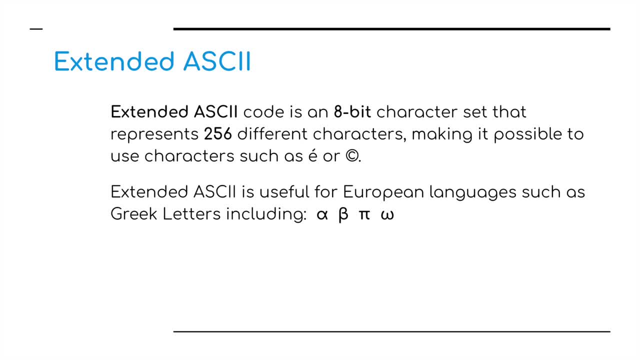 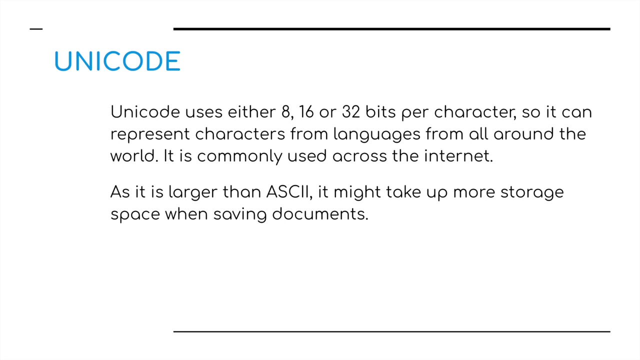 the copyright sign letters with certain accents over them, and various other European languages, such as the Greek alphabet including alpha, beta and pi and and omega. But even with that It wasn't really enough. So a new system was developed, a system called Unicode, which went from 8 to 16 to 32-bit character sets. 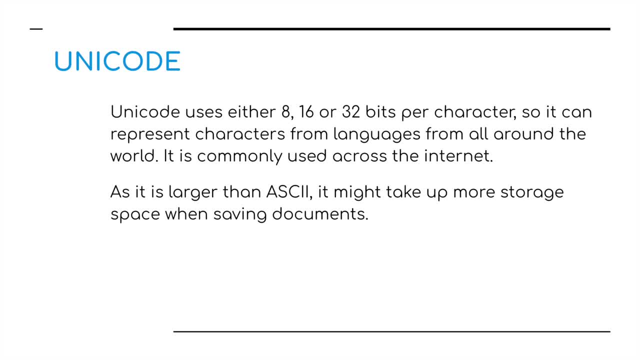 So with 32 bits you can store rather a lot of information. In fact, with 32 bits, as you can see here, we can store over 2 billion different characters with 32 bits. So with this now all the emojis that you're obviously familiar with can be stored as well. 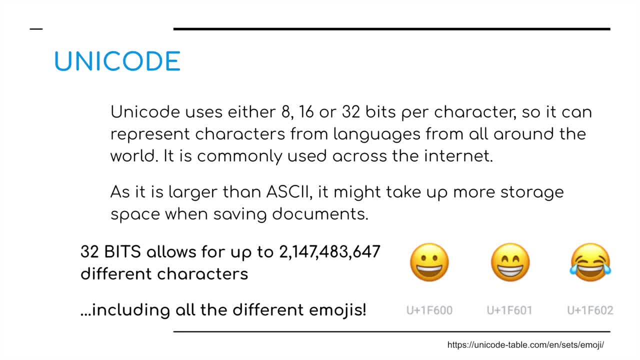 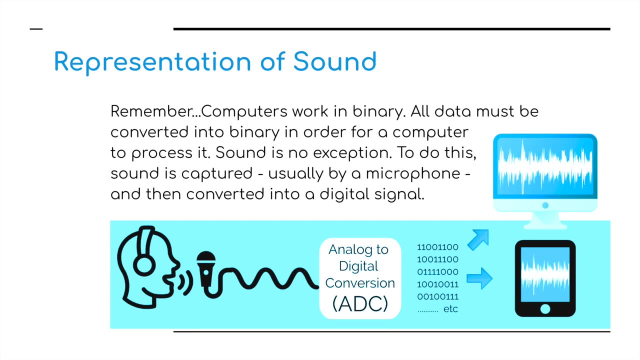 And you can see there, I've used the website unicode-tablecom, a great website for finding out all about Unicode and the various other character sets that are available. Moving on the second part, representation of sound. Now remember, as we said at the very beginning, computers can. 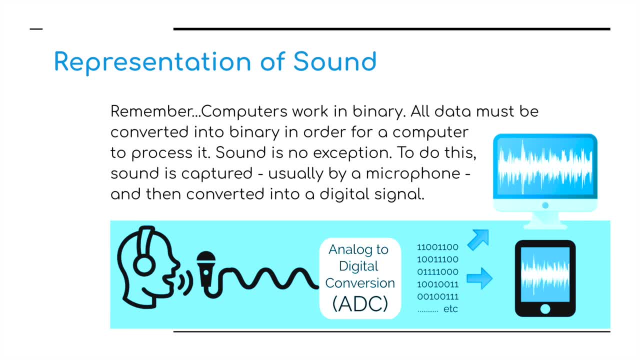 only work in binary. All data must be converted into binary in order for a computer to process it. Sound is of no exception. To do this, sound is captured, usually by a microphone, and then converted into a digital signal. When we speak, when we sing or hear noises, our ears sense vibrations and interpret them as sound. 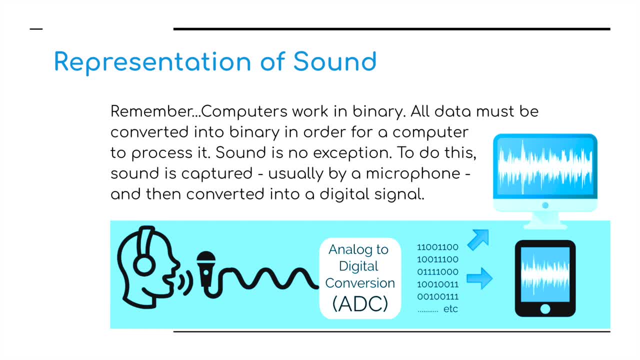 These are what we know as sound waves. Each sound wave has a frequency. Sound waves are measured as a wavelength and an amplitude. The amplitude specifies the loudness of the sound. Sound waves vary continuously. This means that sound is analog. Computers cannot work with analog data, so sound waves need to be sampled in order to be stored in a computer. 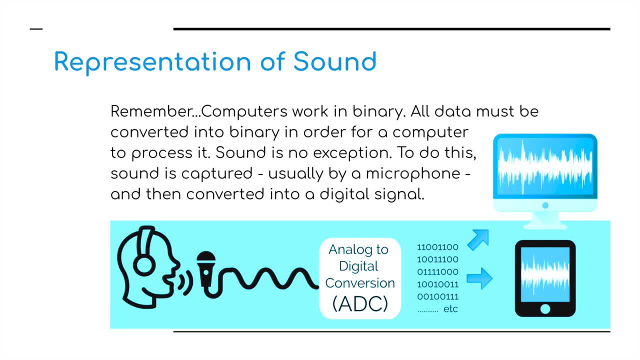 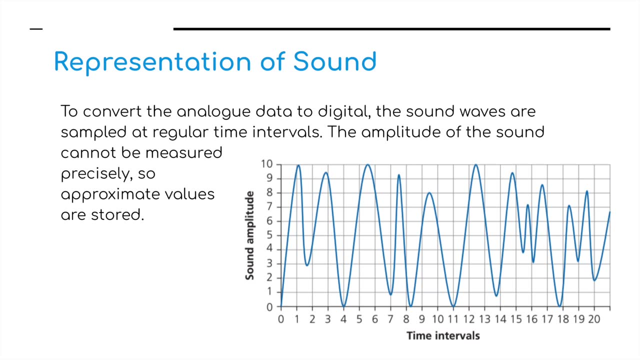 Sampling means measuring the amplitude of a sound wave. This is done using an analog-to-digital converter, As you can see the thing flashing here, something called an ADC- Analog-to-digital converter. Okay, so to convert the analog data to digital, the sound waves are sampled at regular time intervals. 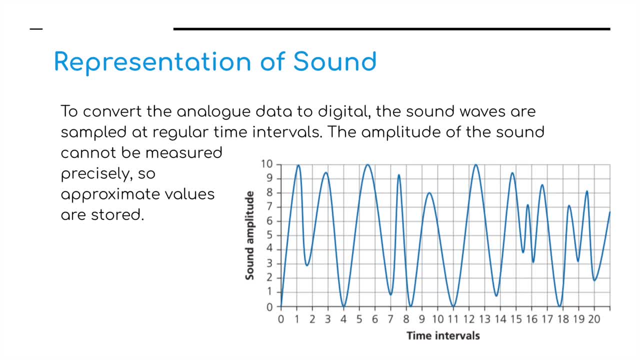 The amplitude of the sound cannot be measured precisely, so approximate values are stored. What does that mean? Well, if we use this graph as an example, the graph shows a sound wave being sampled. The x-axis- the thing along the bottom- shows the time intervals when the sound was sampled. 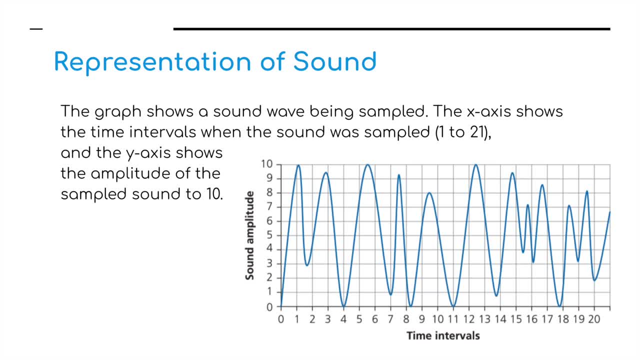 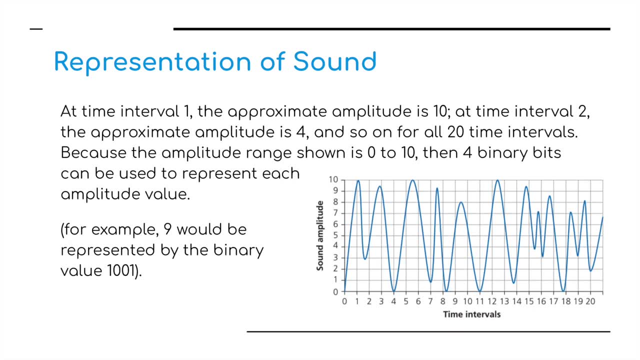 In this case 1 to 21.. And the y-axis shows the amplitude of the sample sound up to 0 to 10.. At time interval 1,- you see here- the approximate amplitude is 10.. At time interval 2, the approximate amplitude is 4.. 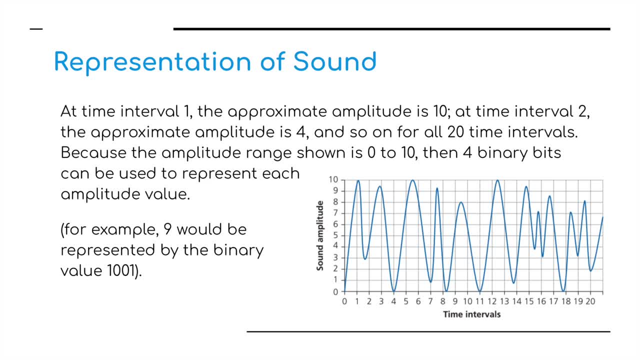 And so on, all 20 time intervals, Because the amplitude range shown is 0 to 10, then 4-bit binary can be used to represent each amplitude value. For example, 9 will be represented, converted to binary, with the value 1001.. 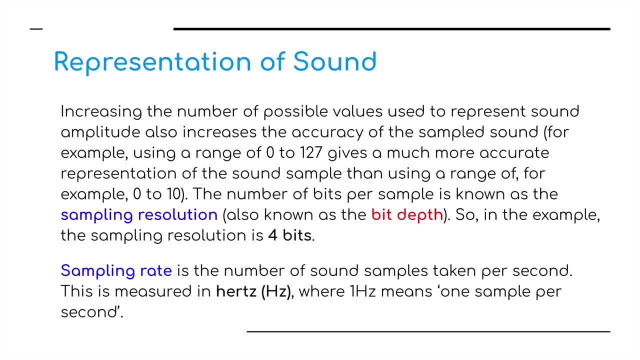 So increasing the number of possible values used to represent sound amplitude also increases the accuracy of the sampled sound. For example, using a range of 0 to 127 gives a much more accurate representation of the sound sample. The number of bits per sample is known as sample resolution, also known as bit depth. 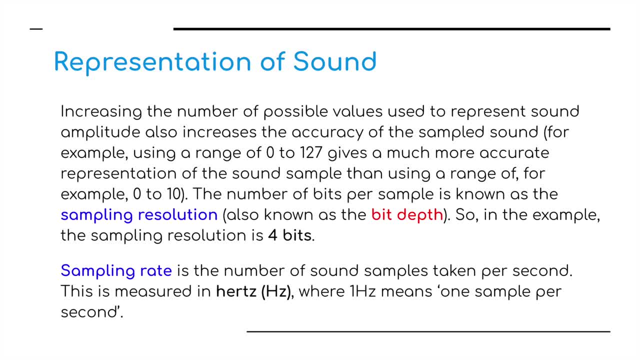 So in the example on the previous slide, the sampling resolution is 4 bits. Sampling rate is the number of sound samples taken per second. This- and you may be familiar with this term- this is measured in hertz. Well, 1 hertz means 1 sample per second. 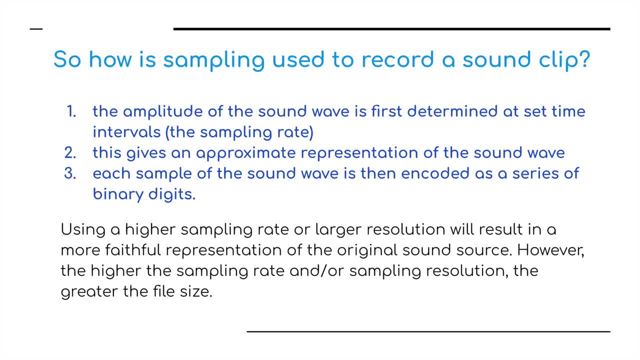 So how is sampling used to record a sound clip? Well, the amplitude of the sound wave is first determined at set time intervals, the sampling rate. This gives an approximate representation of the sound wave, And each sample of the sound wave is then encoded as a series of binary digits. 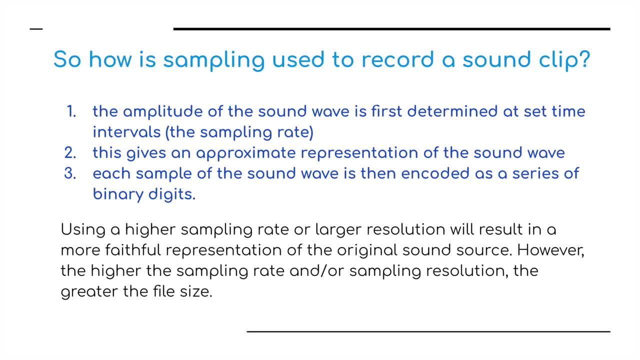 Of course, using a higher sampling rate or larger resolution will result in a more faithful representation of the original sound source. However, the higher the sampling rate and or sampling rate, the greater the file size. So there are obviously benefits and drawbacks of using a larger sampling resolution when recording sound. 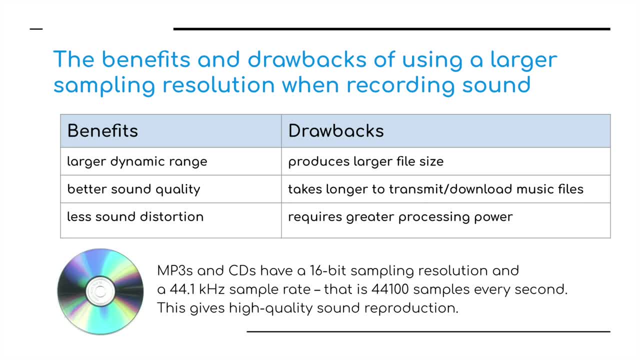 The benefit is obviously much better sound quality, larger dynamic range and less sound distortion, But of course it's going to produce larger file sizes. These large files are going to take longer to transmit or download over the internet And it potentially would require greater processing power. 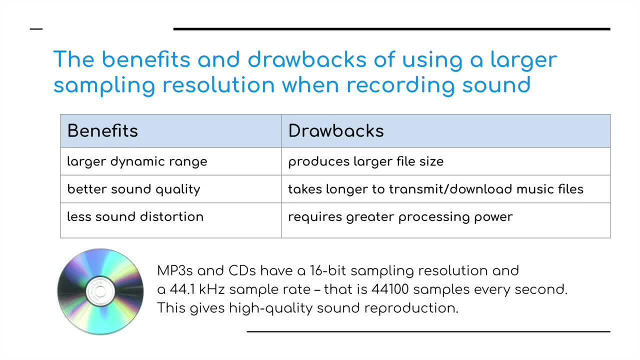 Now there is a standard used generally on MP3s and CDs, And they are sampled using 16-bit sampling resolutions and a 44.1 kilohertz sampling rate. That is, 44,100 samples every second. This being standard gives a very high quality sound reproduction. 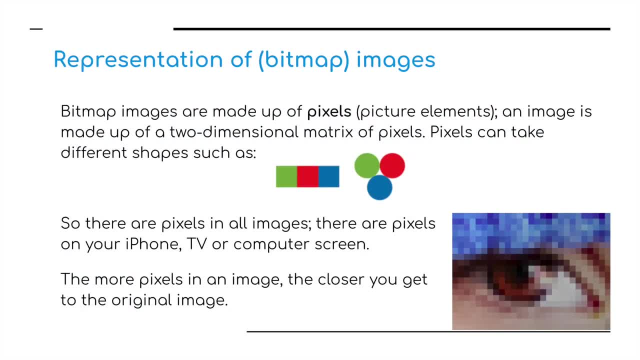 And finally, how do we represent bitmap images on the computer? Well, bitmap images are made up of pixels, a term you may be familiar with. Pixels is short for picture elements. An image, something stored on your computer, is made up of a two-dimensional matrix of pixels. 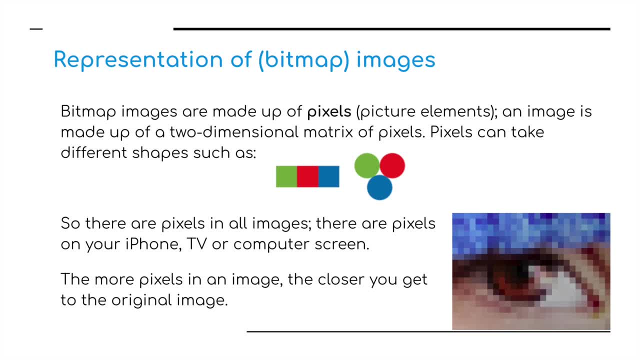 And pixels can take different shapes, such as side by side, in this case, or circles joined together as so. So there are pixels in all images. There are pixels on your iPhone, on your TV screen or on your computer screen. The more pixels in an image, the closer you get to the original image. 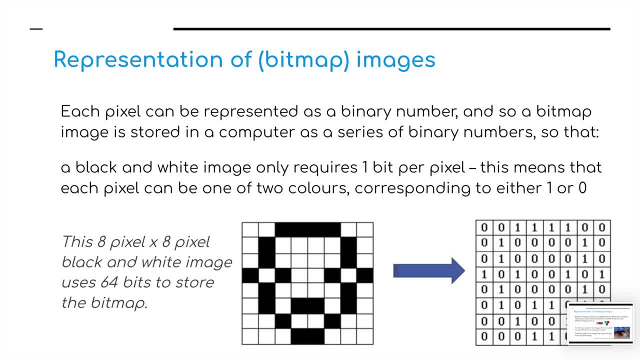 Each pixel, each little tiny square, can be represented as a binary number, And so a bitmap image is stored in a computer as a series of binary numbers, So that, in the example below, a black and white image only requires one bit per pixel to store its information. 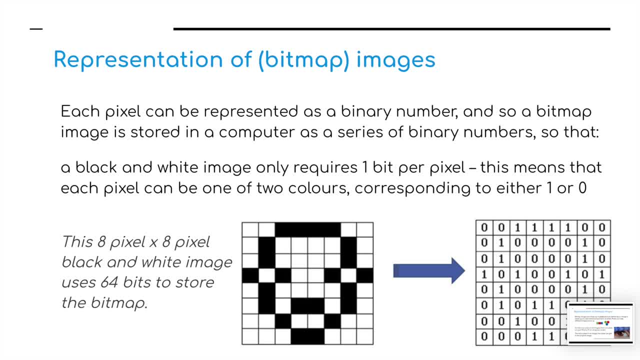 This means that each pixel can be one of two colors corresponding to either a one or a zero. So this little black and white face which we've got on here, an eight by eight pixel grid. black and white image- uses 64 bits to store the bitmap. 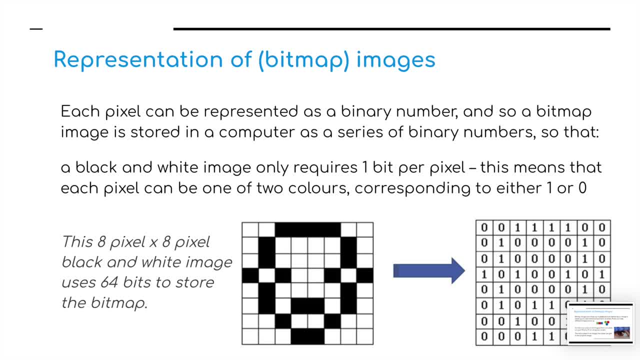 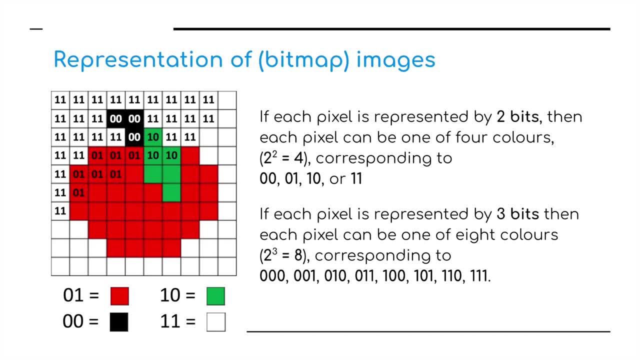 Only zeros and ones. Now, if we want to increase the colors- I'm showing an example here- I've increased it from a one bit, two colors to a two bit image. If each pixel is represented by two bits, then each pixel can be one of four colors. 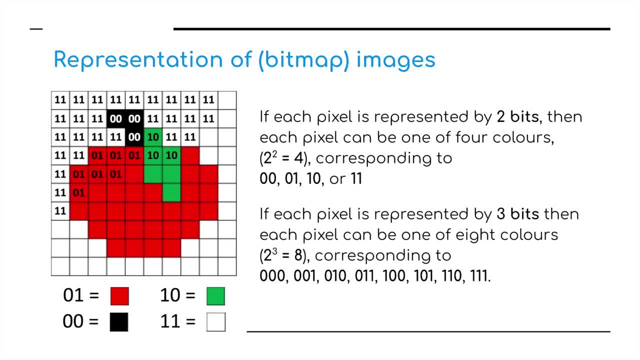 So two to the two equals four, corresponding to the value of zero, zero, Zero, one. one zero or one one. Okay, Obviously this doubles every time. so if each pixel is represented by three bits, then each pixel can be one of eight colors. 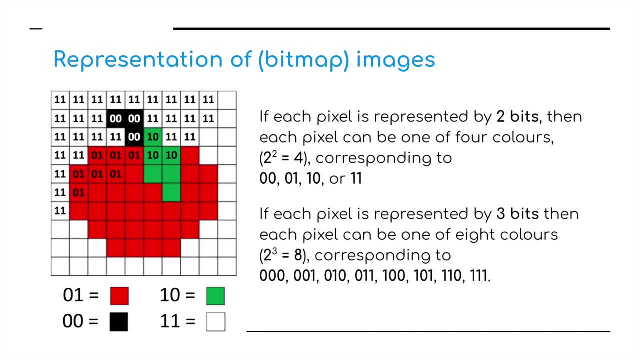 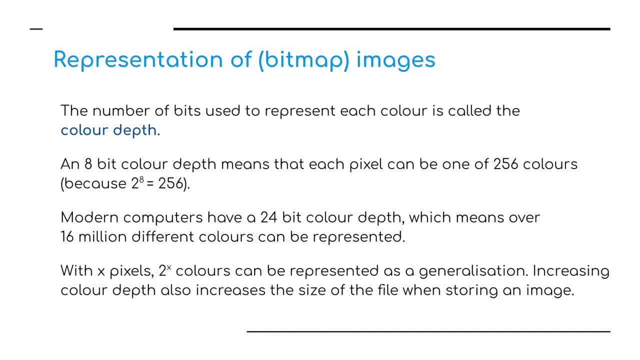 Two to the three equals eight different colors. As you can see there, they would be the corresponding numbers. The number of bits used to represent each color is called the color depth. An eight bit color depth means that each pixel can be one color. 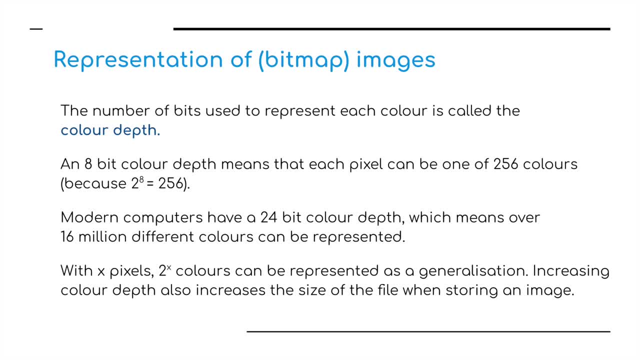 One of 256 different colors. Modern computers, your MacBooks or PC laptops. modern computers have a 24 bit color depth, which means over 60 million different colors can be represented With X pixels. two to the X colors can be represented as a generalization. 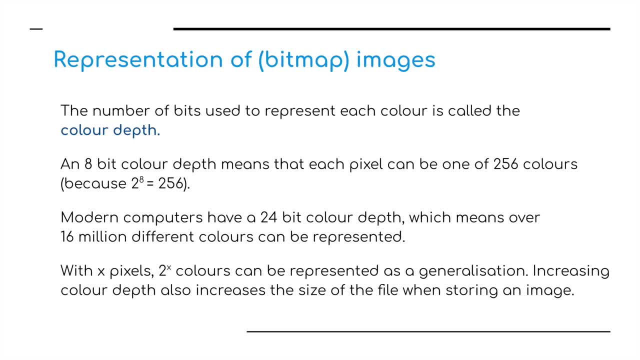 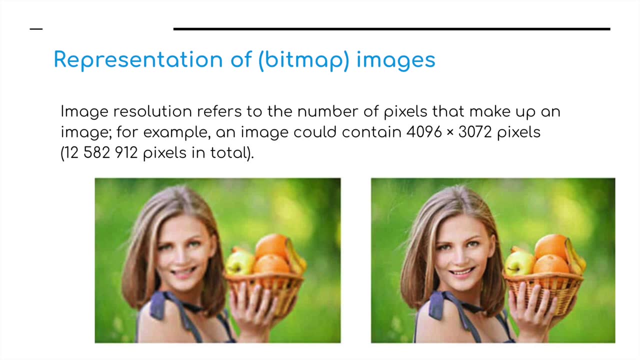 Increasing the color depth also increases the size of the file. when storing an image, Basically like with sound, the better the quality, the bigger the file you're going to need to store. Image resolution refers to the number of pixels that make up an image.